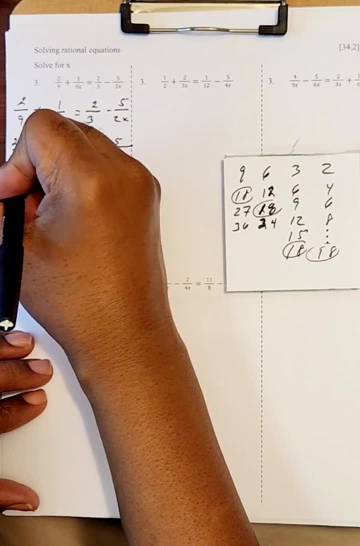 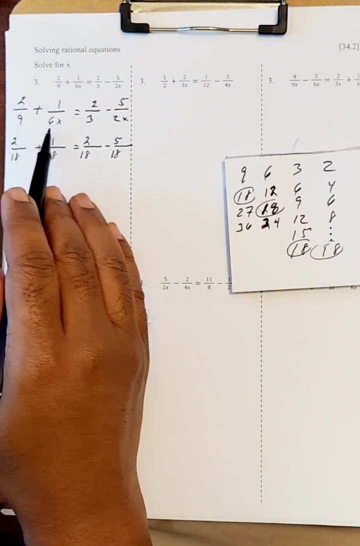 So the common denominator will be 18.. So the common denominator is 18 times 7.. Alright, Okay, so we'll sort that out. The sin number of shit is 3.. Right, But we want to substitute the minus to use the minus again. 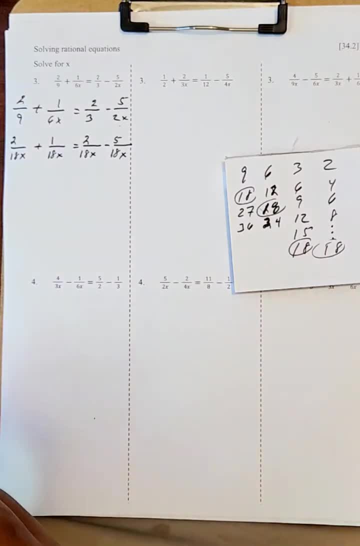 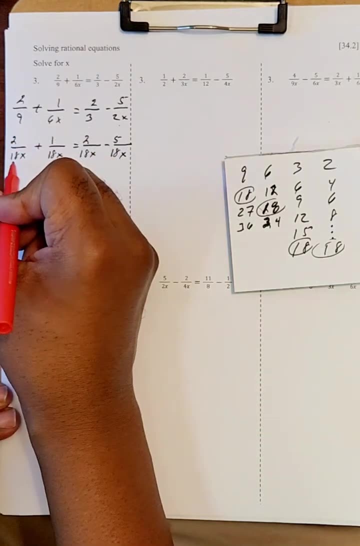 So what we're going to blue is 3.. So now we've got our two, So we're going to put two plus x. Okay, Then we look at the xs, The highest amount of xs we have, x here and x here. 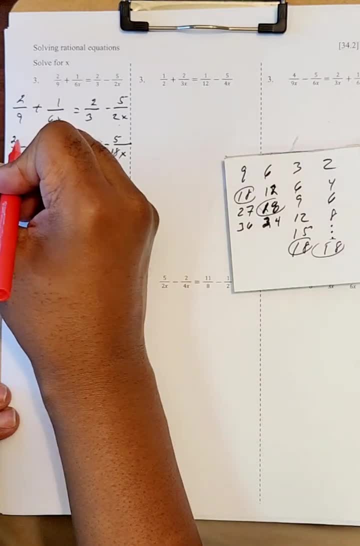 The highest amount of x is x to the first, so we'll put the highest amount of x here, which is x to the first. Alright, That's all. We have our new denominator. Now let's see the difference between our old denominators and our new denominators. 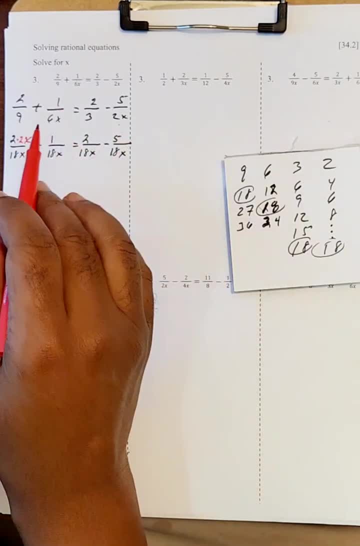 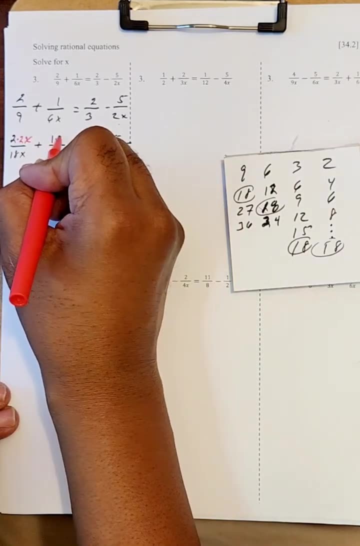 between a no x and an x is an x. okay, the difference between a 6 and a 18. the factor between a 6 and 18 is 3, so there's a times 3 in there, and the difference between having an x and having an x. 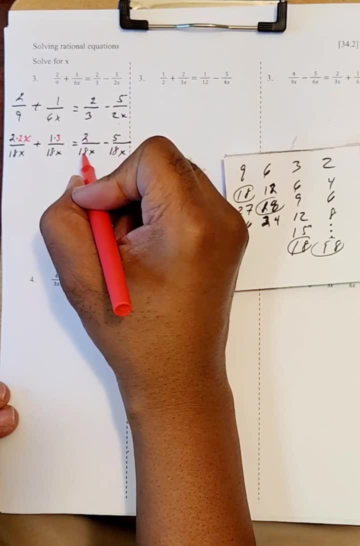 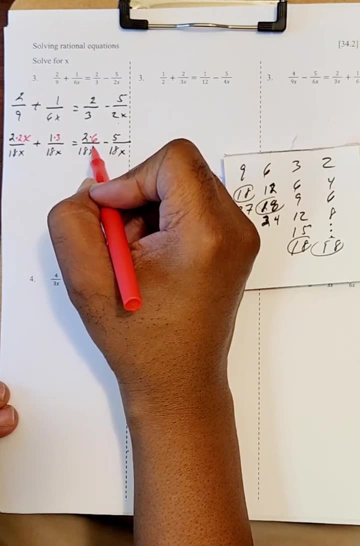 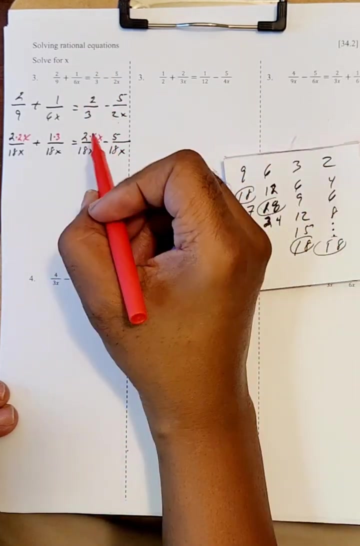 is no difference. so there. so the difference between having a 3 and an 18 is multiplying by 6, so we'll multiply this by 6 and we and we don't have an x, and now we have an x, so an x has been added, so we'll have to add an x there and finally, here there's going to be a 2 and 18 is 9, so this: 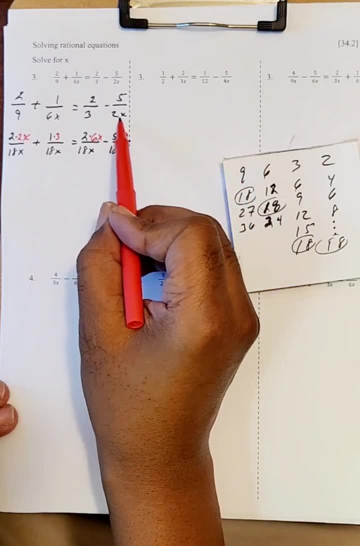 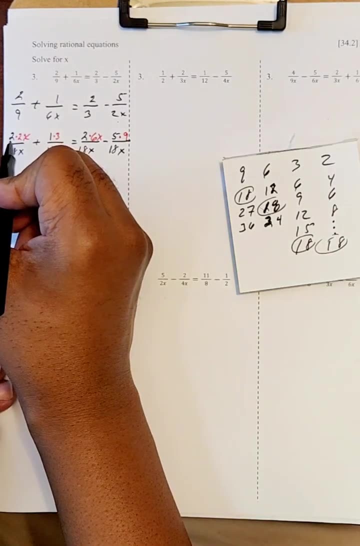 would be 5 times 9, and there's no. there's an x here and there's an x there, so there's no x added. now let's go gather our numerators. the 2 times 2x will be a 4x, plus 1 times 3 will be a 3. 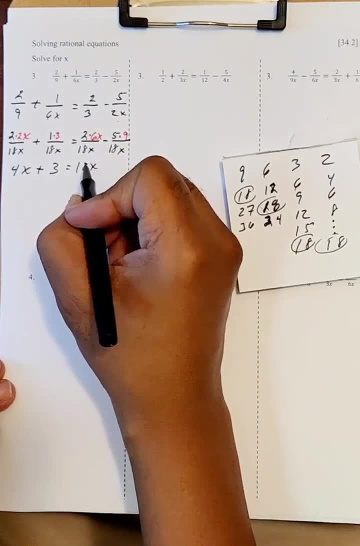 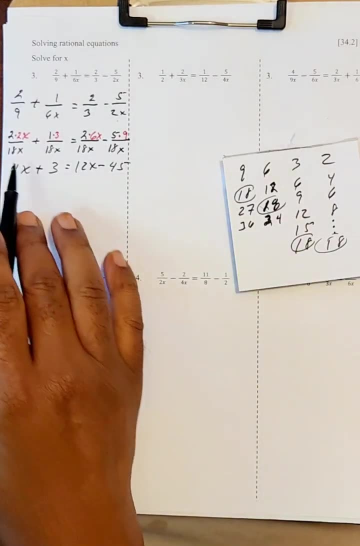 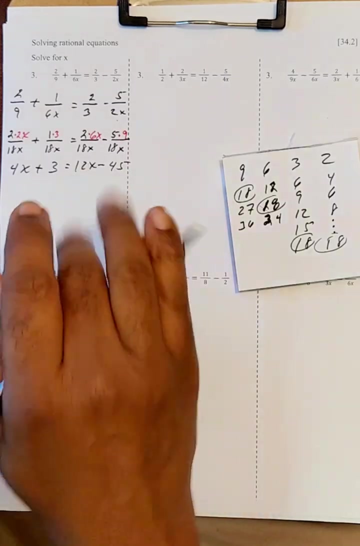 2 times 6x will be a 12x and minus 5 times 9 is going to be a 45, and we don't have to write our denominators, since they're all common. we just need our numerators. so solving here I'm going to take. I want my x's to be on this side, so we'll. 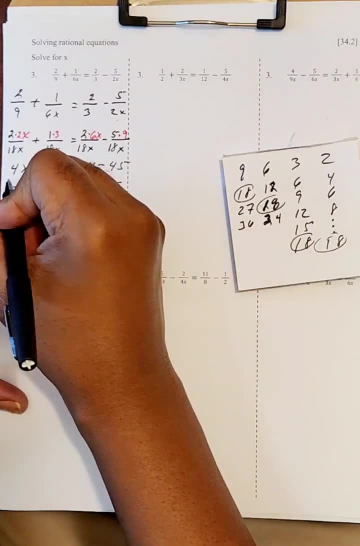 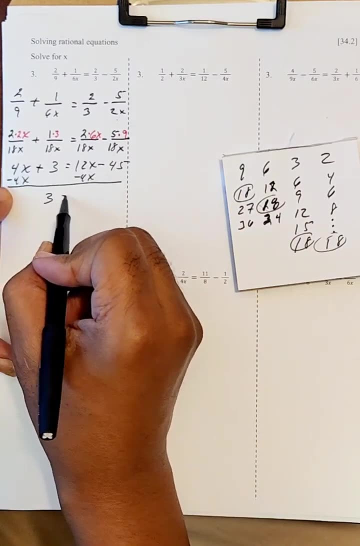 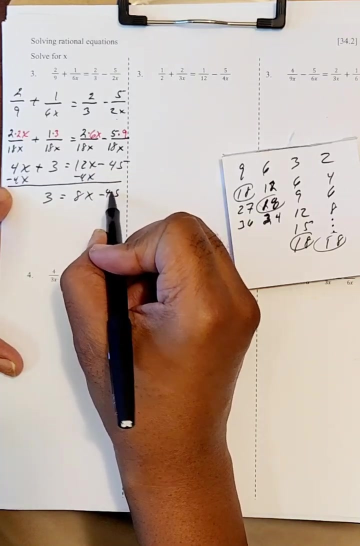 get rid of the adding 4x by using a subtracting 4x here and then here, and so the x's cancel out and we get 3 equals 12x minus 4x leaves me with 8x's. and then there's the minus 45's. 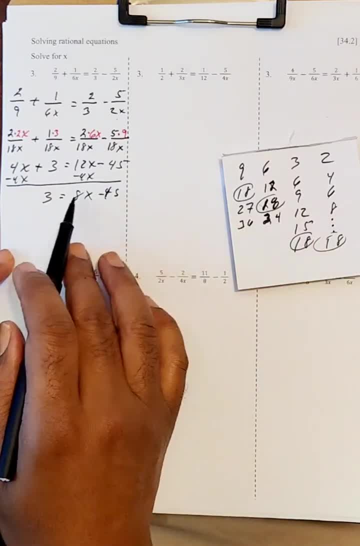 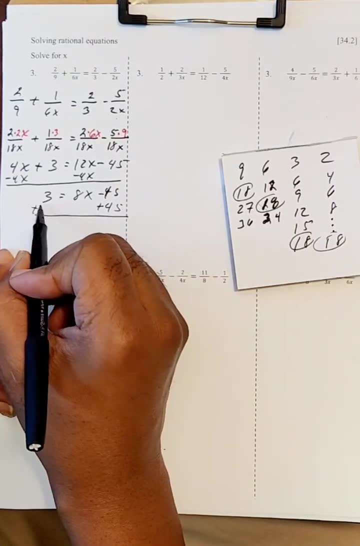 now I want to get rid of the minus 45, and then the 8, and then I'll have my x isolated. so to get rid of the minus 45, I'm going to say a plus 45 here, then a plus 45 here, and this is going to give me 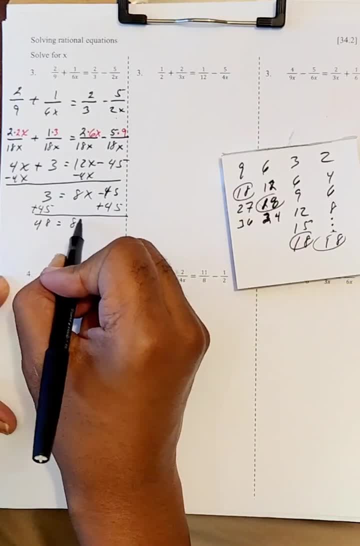 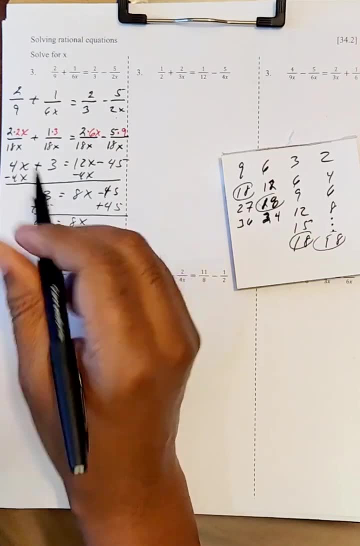 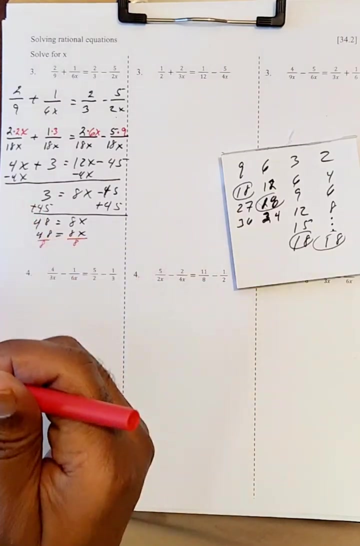 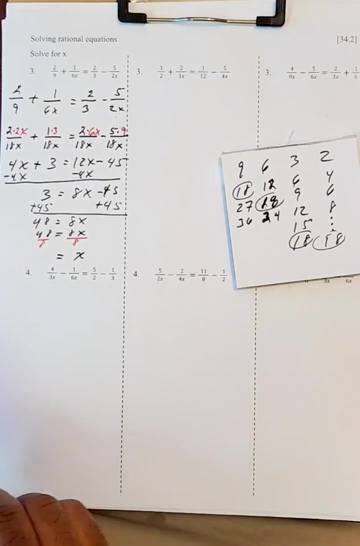 48 here equals 8x and this is going to cancel here. now we're going to take our 48 equals 8x and divide by 8 on both sides, okay, so dividing by 8 gives me an x, and 48 divided by 8- that divides evenly, that is a 6. 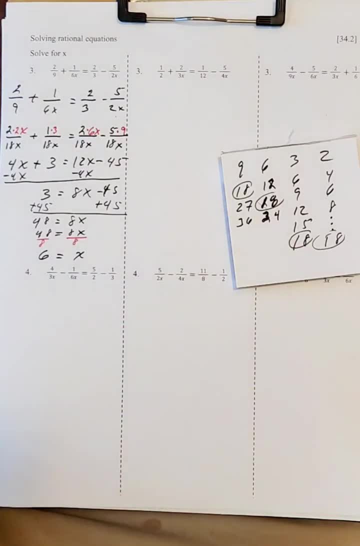 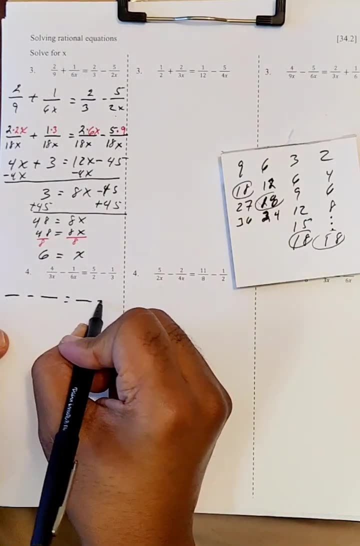 because 6 times 8 is 48, so the solution is x. all right, let's try the next one. the next one: we have a fraction minus a fraction equals a fraction minus a fraction. our numerators are 4, 1, 5 and 1. 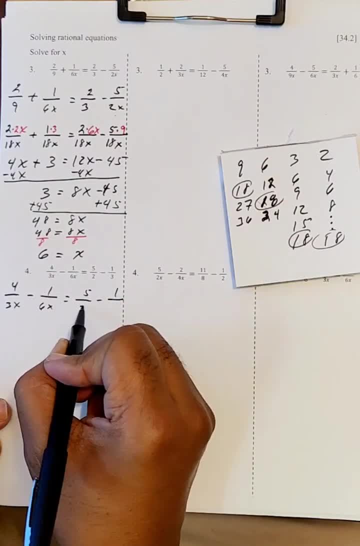 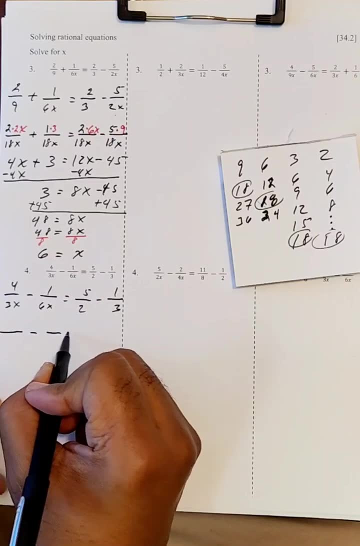 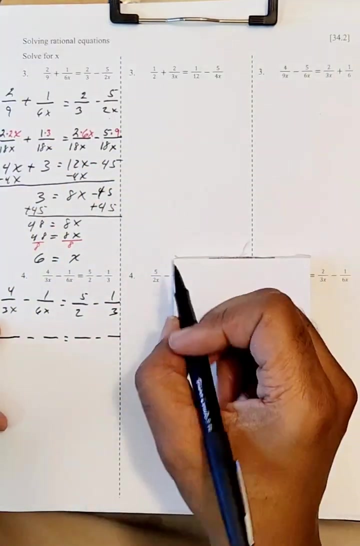 denominators are 3x, 6x, 2 and a 3. okay, so let's create new fractions, all with the same denominators. okay, let's get rid of this paper here. all right, our denominators are 3, 6, 2 and 3. so what's going? 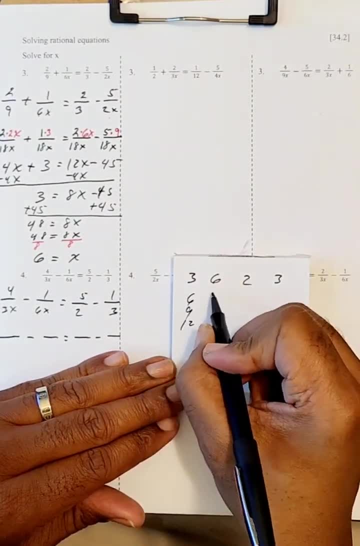 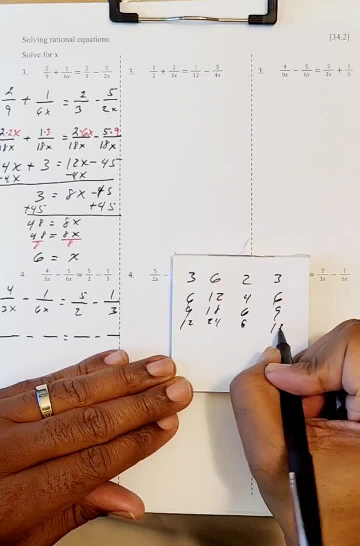 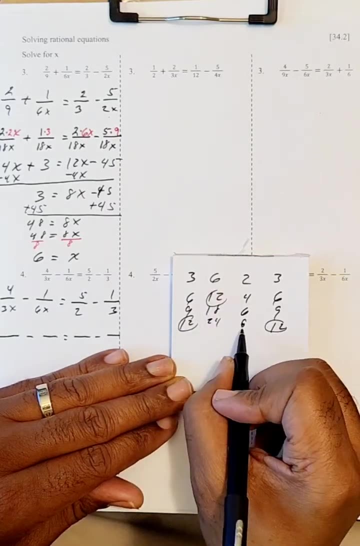 6, 8 and 3, 6, 9, 12. well, i'm already seeing a pattern. i'm already seeing a 12 develop here, here and here. so i'm so i'm going to take this one right here down to a 12 as well. so we have 12s everywhere. 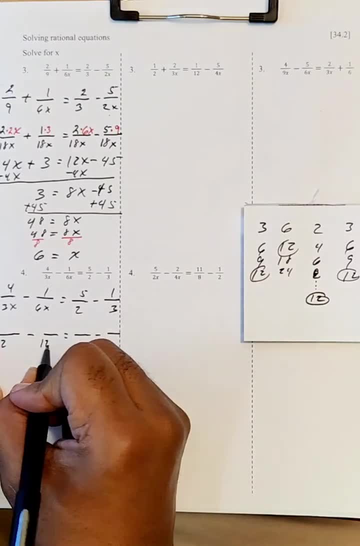 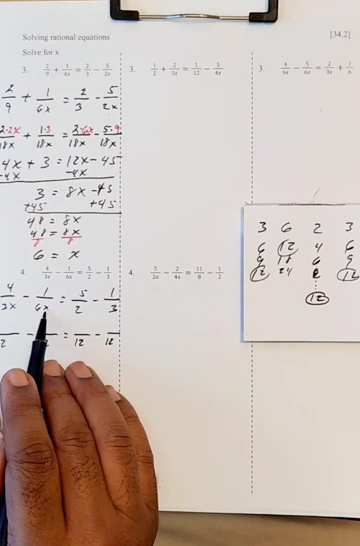 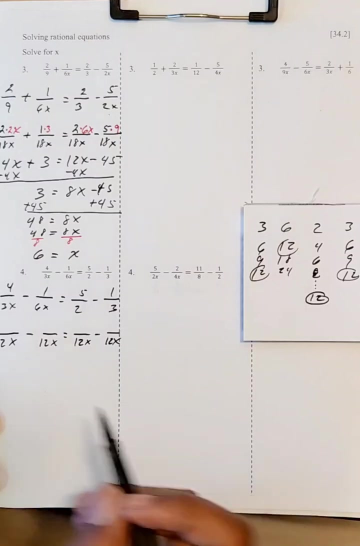 so the denominators all have 12 all right. now for the x's. this is: this is 1x or x to the first power. this is x to the first power. so the highest amount of x is around here- x to the first power. so everybody gets the x to the first power now. the numerators are 4, 1, 5 and 1. let's see what we. 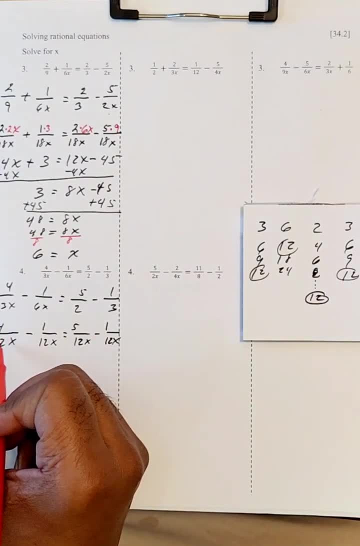 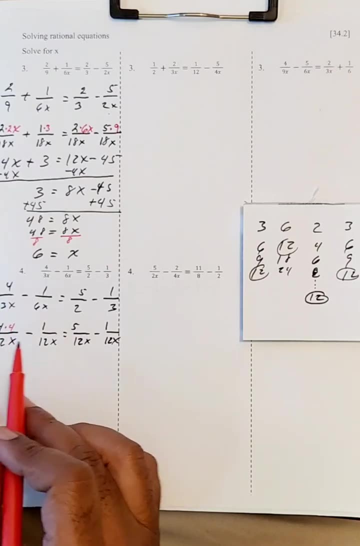 need to do. the difference between having a 3 and a 12 is that um there's an additional 4 here, so we multiply by 4. there's an x there. there's an x. there are no changes on the distance to a 6 and a. 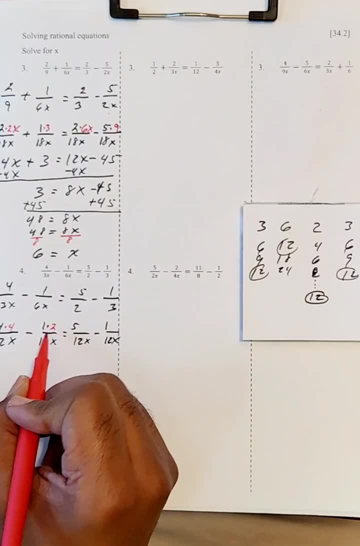 12 is multiplied by 2, so we need an extra 2 here, since there's an extra 2 in the denominator and we need no more x's because there's an x there, so we need an extra 2 here. so we need an extra 2. 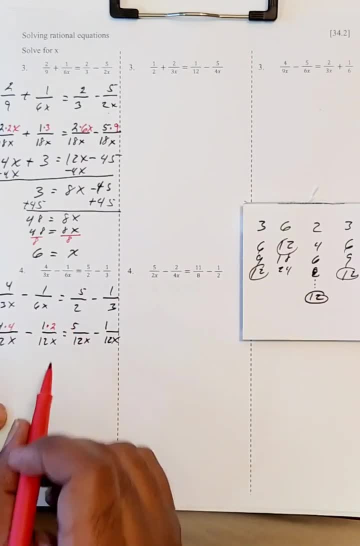 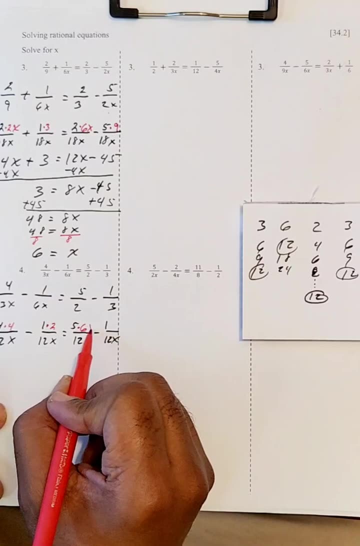 there the x there. the difference between a 2 and a 12 here is 6, so we'll make this times 6. now there's no x here and there is an x here, so x has been included. so we'll include the x in the. 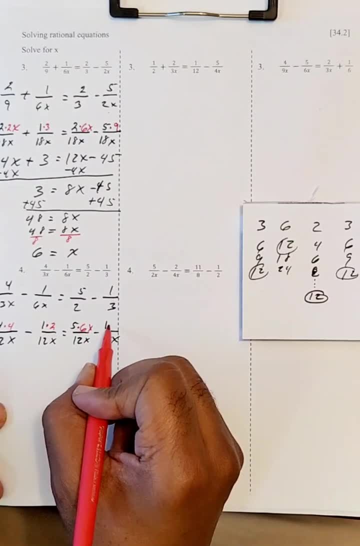 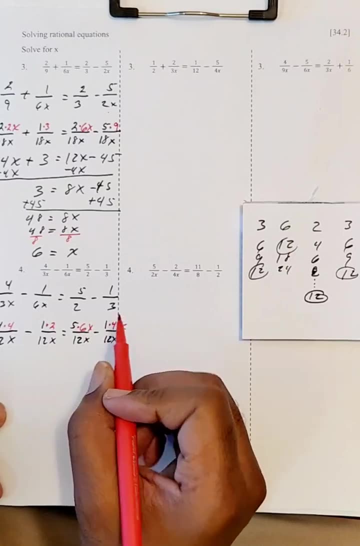 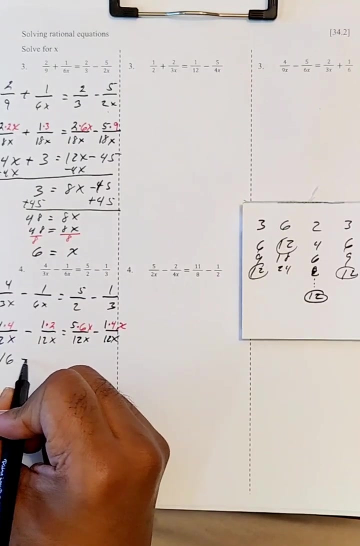 numerator and the difference between a 3 and a 12 is 4, so it'd be a times 4 and there's no x here. there is an x in this denominator, so extra x has been included, so let's add another x there. so our numerators are now 4 times 4, 16 minus 1. 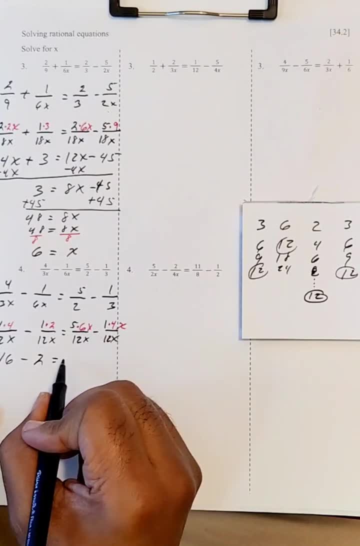 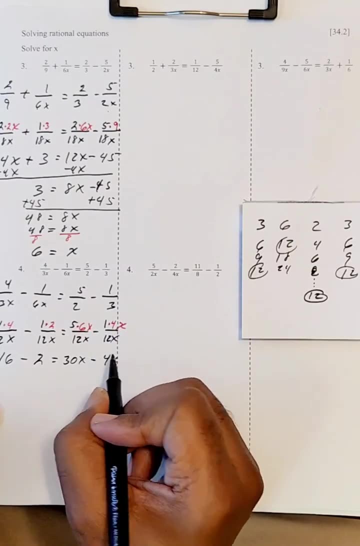 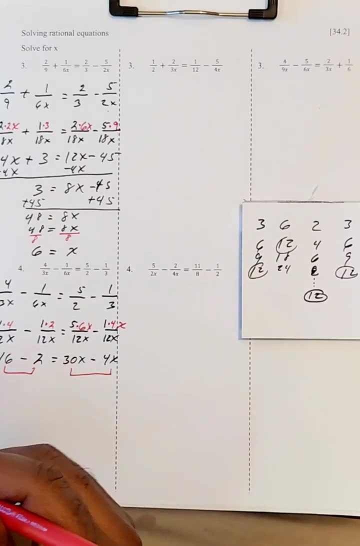 times 2, which is 2, 5 times 6x, which is 30x, and minus 1 times 4x, which is going to be 4x. now we can combine like terms. these are like terms here and these are like terms. so if i combine the 16 and the,